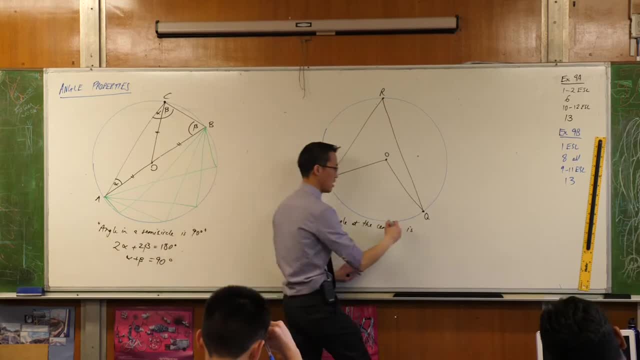 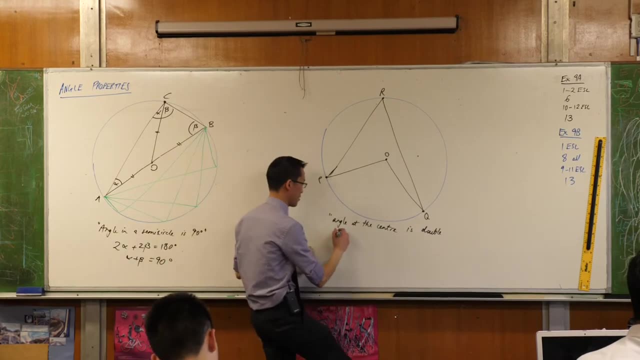 is Nadir. you said double, right Double- You could say twice, but double is fine as well- Is double the angle at the circumference, and even though I think that's sort of enough to unambiguously within this context, 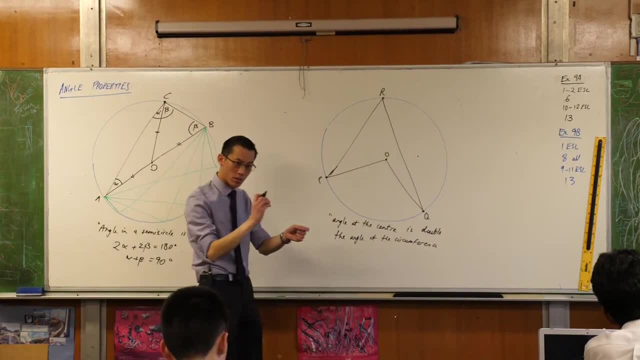 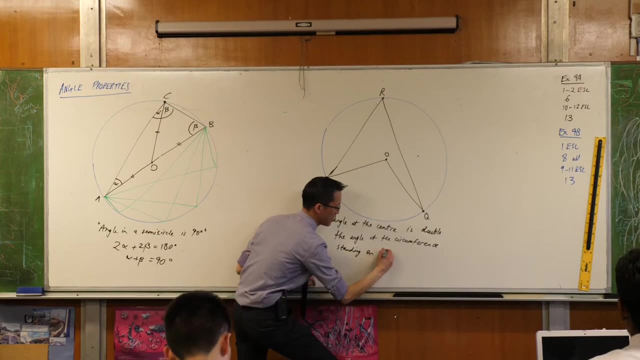 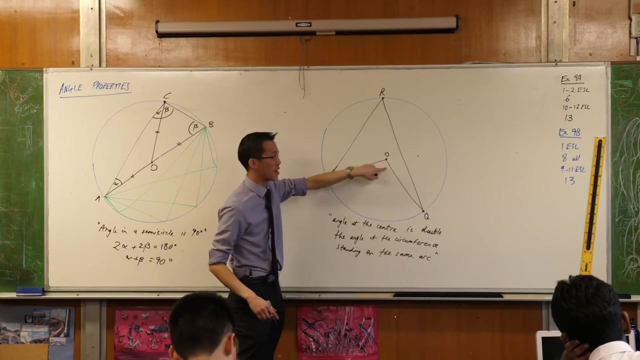 describe what you're talking about. I think it's a little more descriptive to add one more phrase at the end, which is standing on the same arc, Because that's how we constructed these, remember. So what we're suggesting is this angle, twice the size of this one. 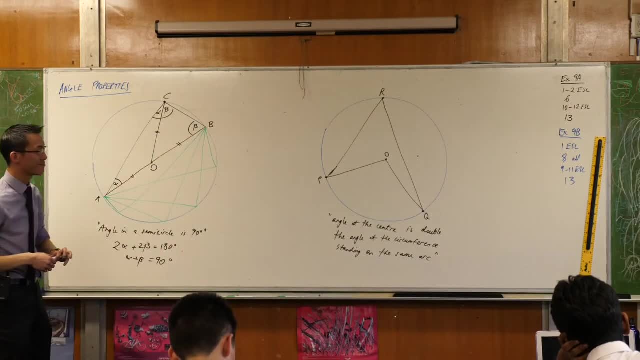 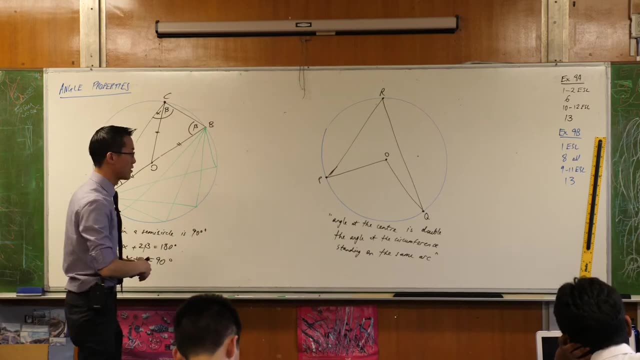 Eric, What if R is somewhere else? that doesn't make that nice little thingy shape where it's? you know, so much across the Yep. yeah, yeah, yeah. That is a great question. If, for example, 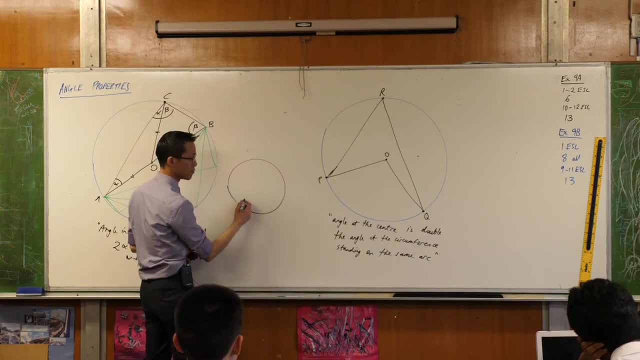 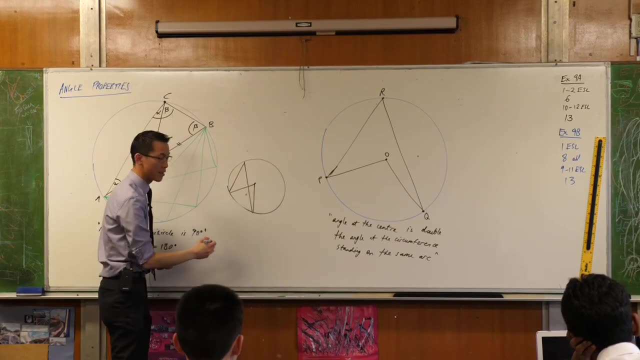 I'll just draw one over here. that's not the centre, that's the centre. So say something like this, for instance, like that: yeah, So one of the wonderful things about this and the reason why I've stated it in this way, 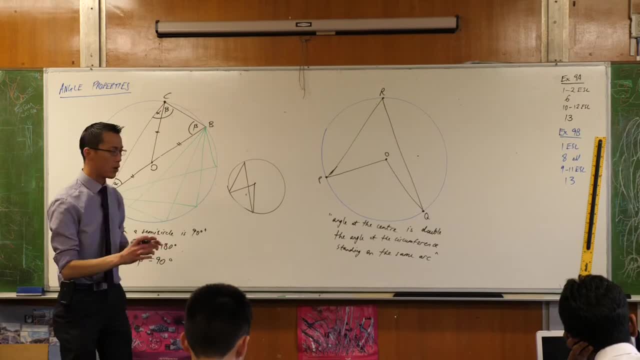 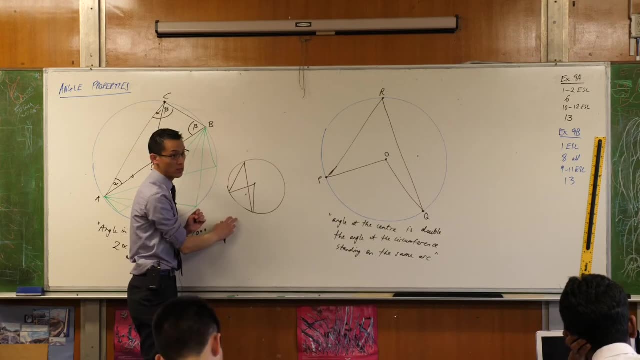 is that this is still true. It's still true. The proof that we'll use will end up being slightly different because, as you can see, these do look like different configurations, don't they? But we can still do it just as well as we can do it over here. 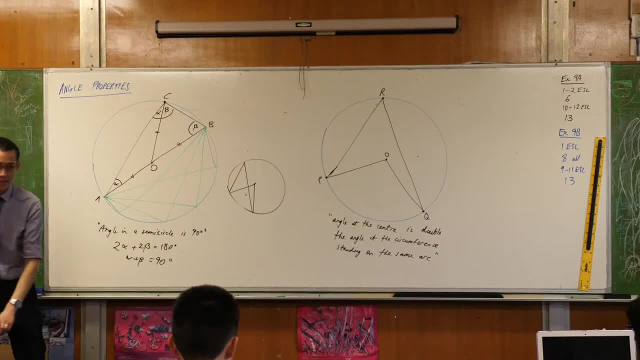 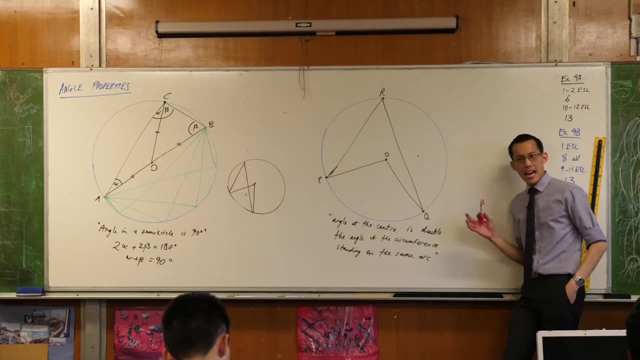 So again, I'm going to try and walk you through. I'll let you have a one minute head start this time, because this time I just sort of gave it to you, maybe two minutes. I'm generous If what we're trying to prove. 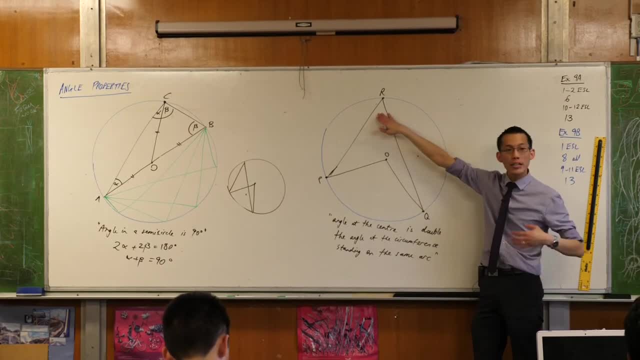 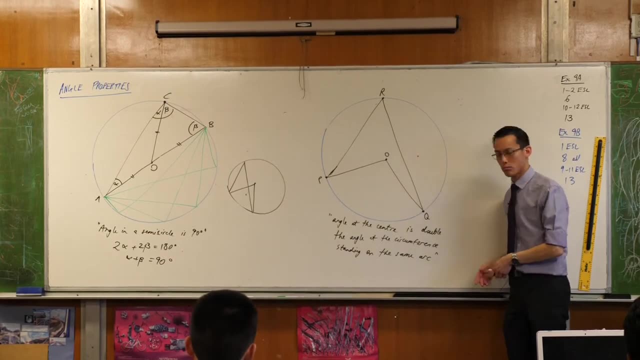 is that this angle is double this angle, and I've already suggested to you that within circles, constructions are often very, very helpful. What could you do to get towards something like this? Just draw something, nothing is wrong, but obviously when you start to put too many drawings on there, 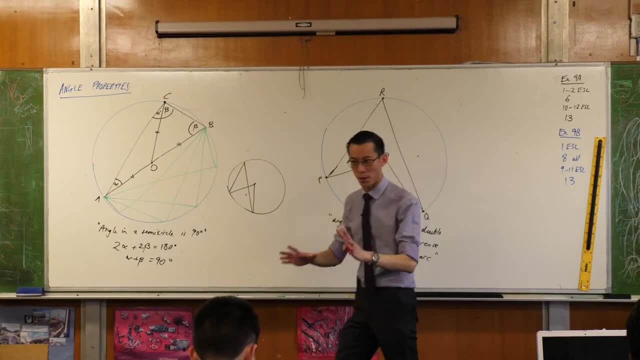 it just gets clouded. If you think you've got something, call me over. I don't want to spoil it for everyone, so have a shot. All right, it's perfectly fine if you're not done yet. The point of this is not necessarily to get the answer. 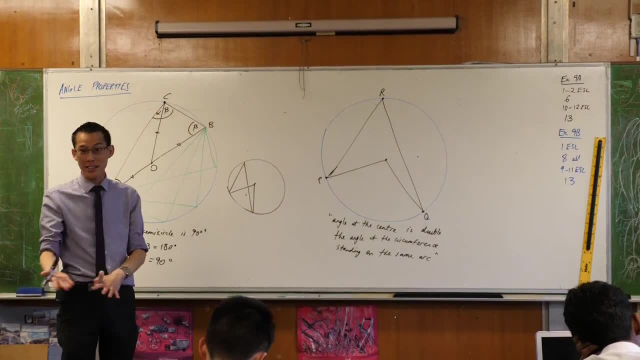 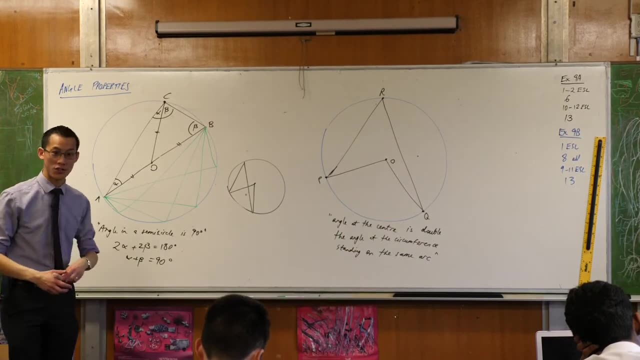 but to stretch your muscles and think geometrically It's quite different to doing, say, calculus, right? Okay, I'm just going to shuffle this over a little bit because I'm going to make a construction Now. like I said, 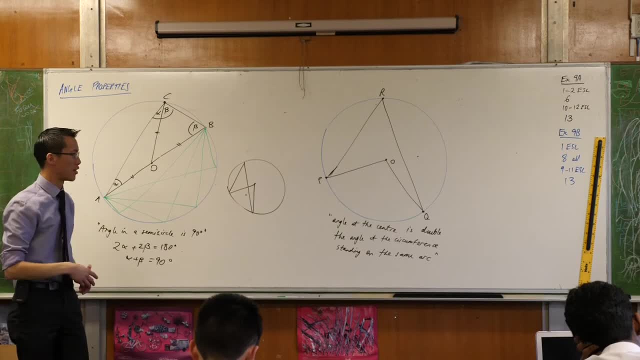 there's a few different ways to do this, lots and lots of ways to do this. Eric just showed me one that I'm going to come to in a second. I'm going to show you my preferred proof, because I think it's quite nice and quick. 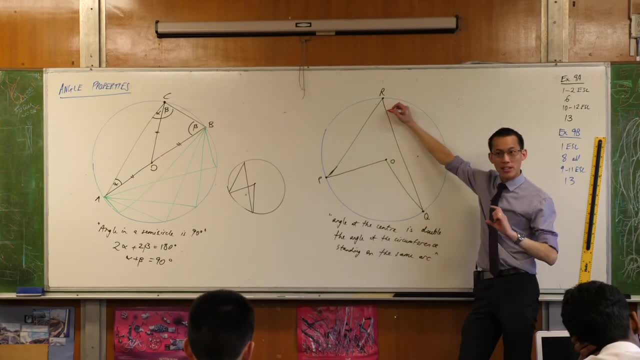 It's only minor difference. Okay, I made a construction RO, but I didn't construct the radius. I actually went a little bit further. You don't have to go much further. you don't even have to go to the opposite side of the circle. 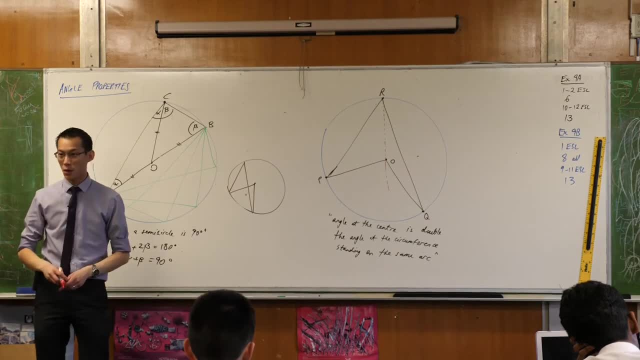 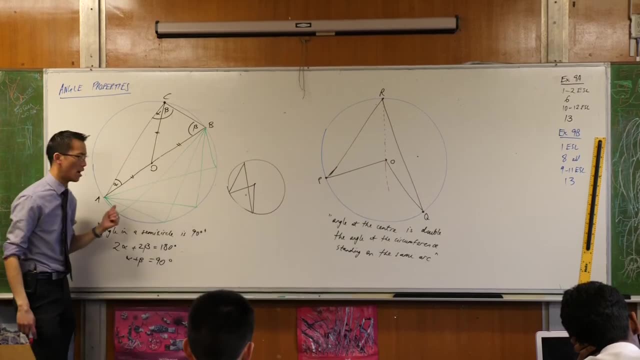 You just have to go past the centre. Here's what I'm going to do. Having done that, you've got- maybe you see it right, You've got- the same situation here as you do over here, in that you've got all these isosceles triangles magically appearing. 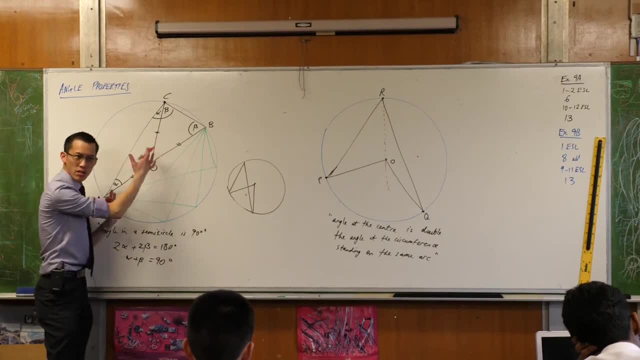 Are you getting a hint? yet In circles you get lots of isosceles triangles because you have radii everywhere, So they're very easy to find. So for that reason- just like over there, if I have a look at say, 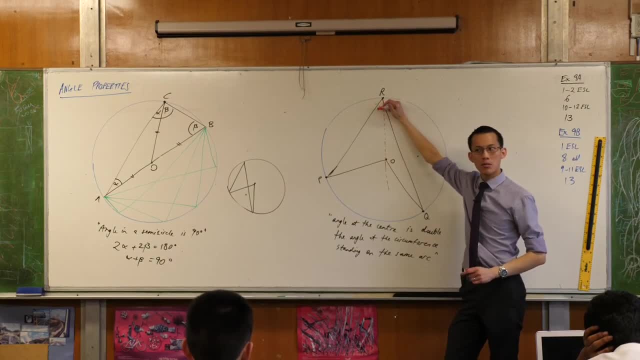 this angle up the top. it's going to be equal to have. I got enough names on here. I do. Can you tell me the name of the angle? it's equal to RPO, right? Because here are the radii. 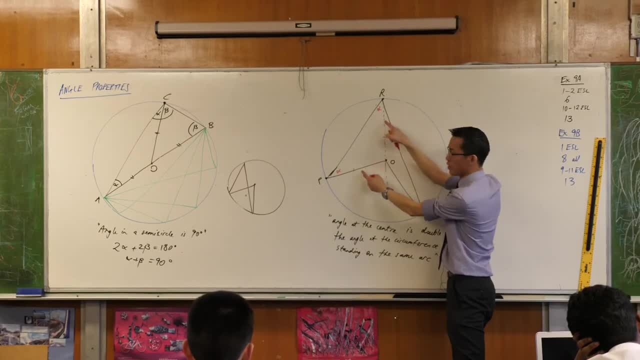 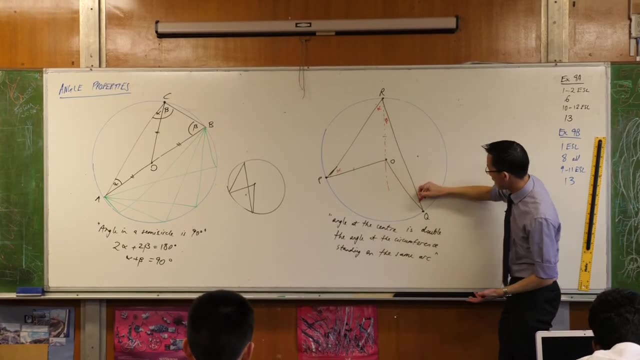 and so equal angles are opposite equal sides. Yep, By the same logic, I can look at this thin triangle over here, and if this is beta, then this guy down here is also beta. Okay, Now you have a couple of choices from here. 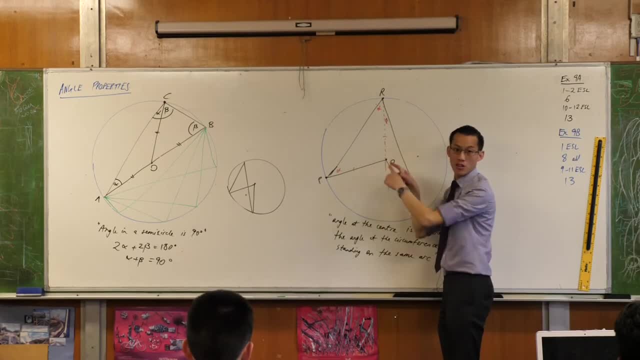 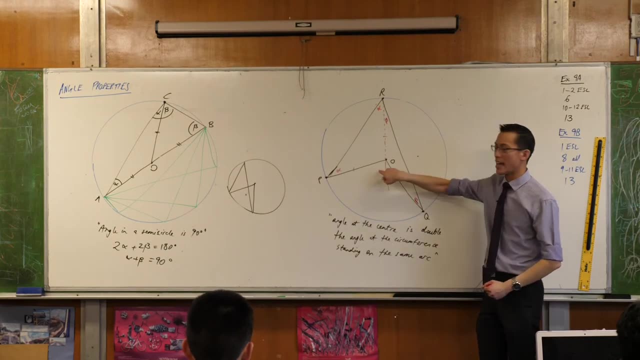 I know where Eric went is that he went to these angles inside the triangles, which is perfectly fine. You can find out what they are angles on the triangle- But there's an even more direct way to get to this angle that I'm interested in, right. 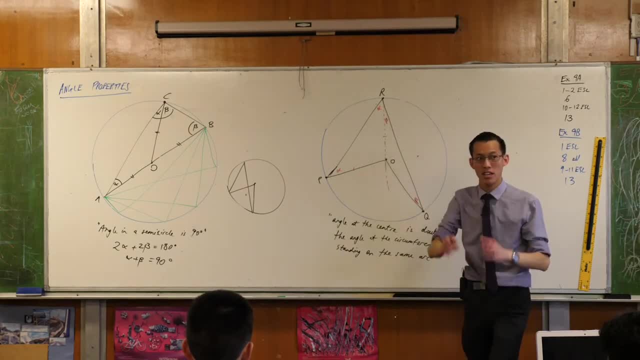 By the way, I've called this angle alpha and this angle beta. So, in theory, what should this angle be equal to? If my property is right, what should it be equal to? It should be equal to exactly double alpha plus beta. 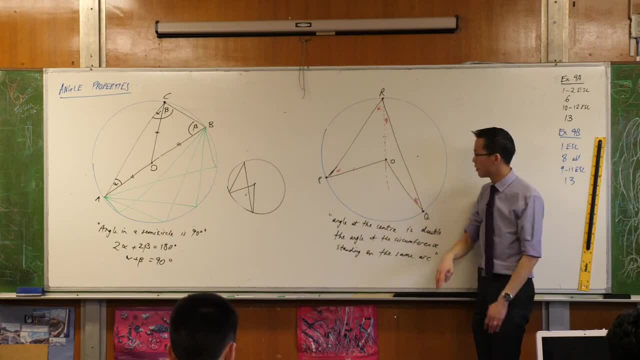 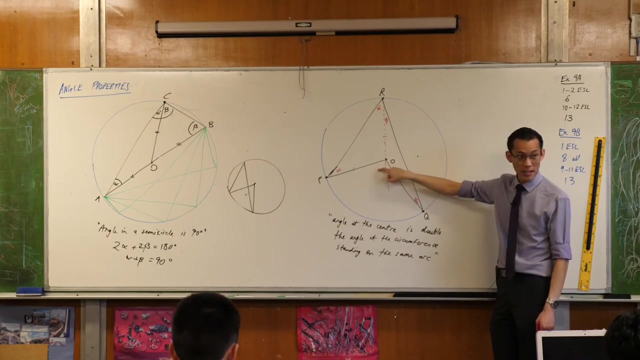 which is 2 alpha plus 2 beta. You agree, Watch Angles, they're related to this one. What's the relationship between alpha and alpha and this guy right here, This one in here, this one in here? I'll give you a clue.